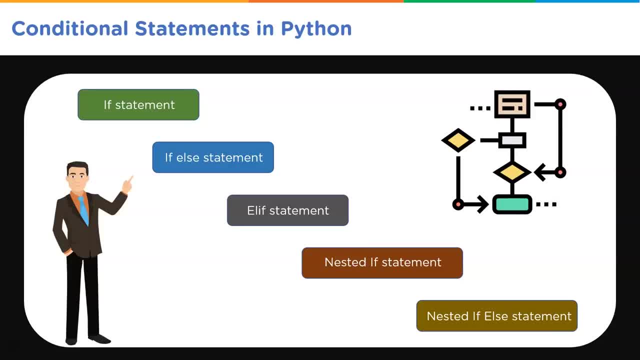 actions depending on whether a specific Boolean constant evaluates to true or false. Conditional statements are handled by blocks of if statements in Python. Now conditional statements are also known as decision-making statements. So Python provides different types of conditional statements that you can use to make decisions. We have the simple if statement, Then we have if-else statement. 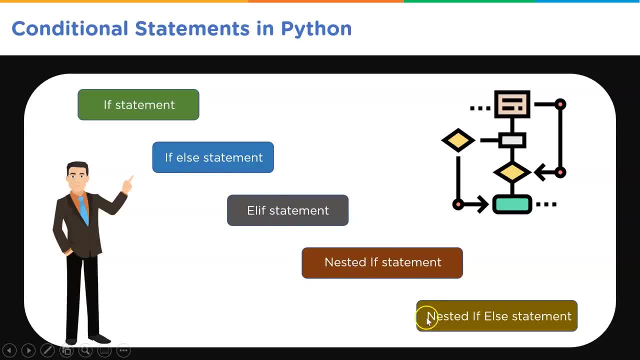 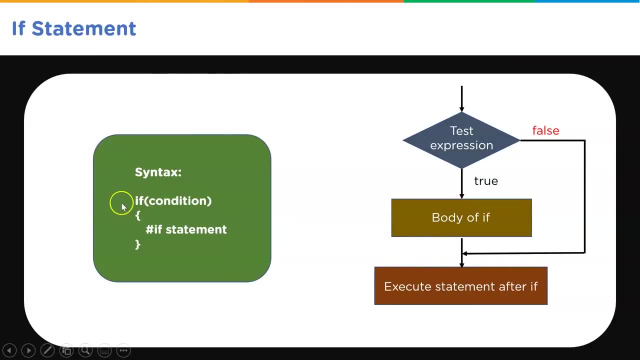 elif statement, the nested if statement, as well as nested if-else statement. We will learn them one by one with the help of their syntax and code examples. So this is how the syntax of if statement looks like. So you pass in the if condition and then. 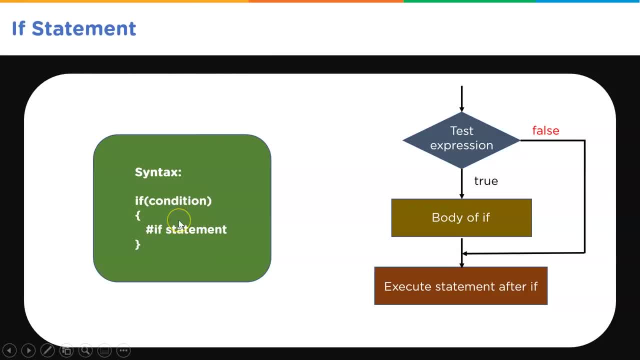 we have a set of statements inside the if condition. So on the right side you can see the flow diagram, how the if statement gets evaluated. So first we have the test expression. now, if this expression evaluates to true, then we go inside the body of the if statement. 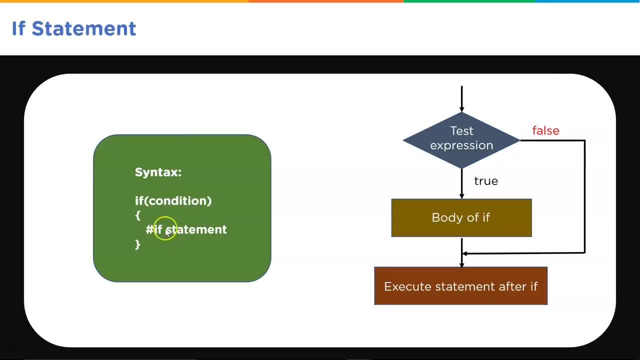 So this is basically the body of the if statement that contains a list of statements or blocks of statements. Now, if the test expression evaluates to false, we execute the statements that are present after the if condition. Alright, now let me take you to my Jupyter Notebook. 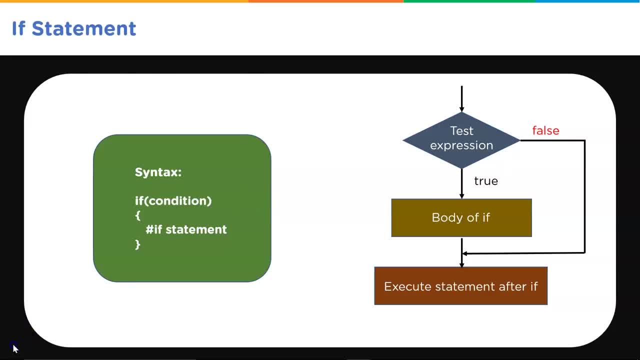 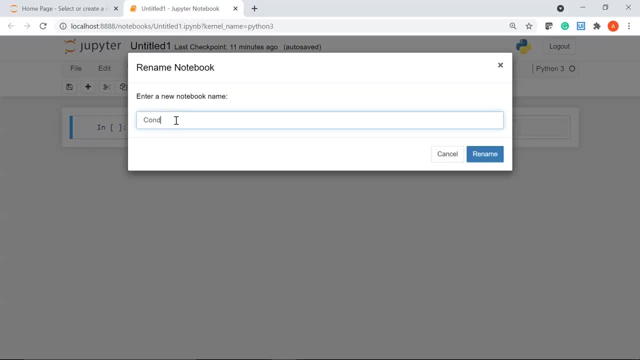 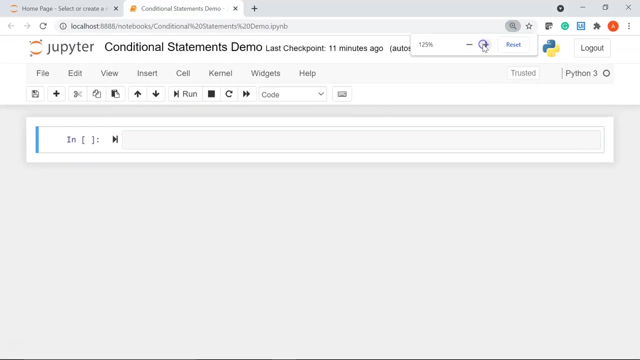 to understand if statement with an example. Okay. so here I am on my Jupyter Notebook. I'll just rename this to conditional statements. I'll see it as demo and we'll rename it. Okay. I'll just expand the screen size, Alright, okay. So first of all, I'm going to create 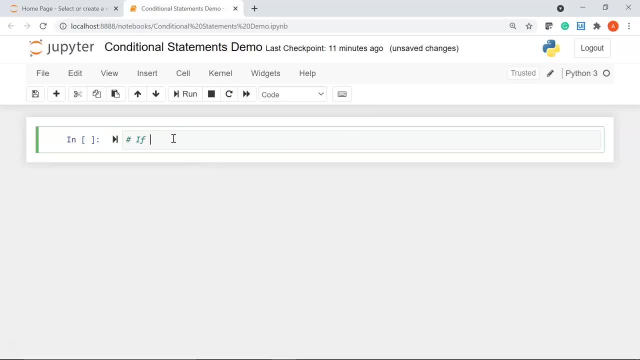 a statement. Let's write a simple if statement. I have given a comment here. Suppose we have a variable called grade and the value of grade is 80. Then I'll write my if statement as if Grade is greater than equal to 50. Then I'll give a comment here. Let's write a simple. 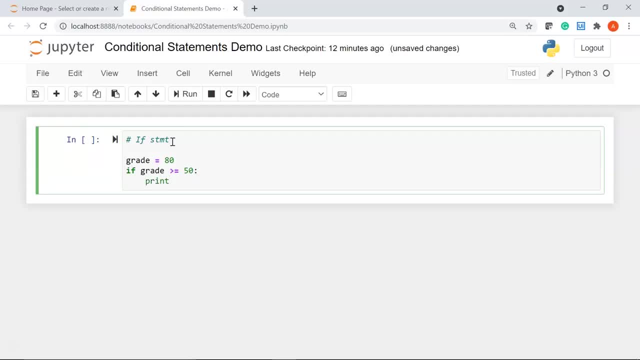 if statement colon. Then I'll write a print statement. Print passed in the exam. Now this is how you write a simple if statement. So you have the if keyword followed by the condition. So here my condition is: I'm checking whether the grade is greater than equal to 50.. Now 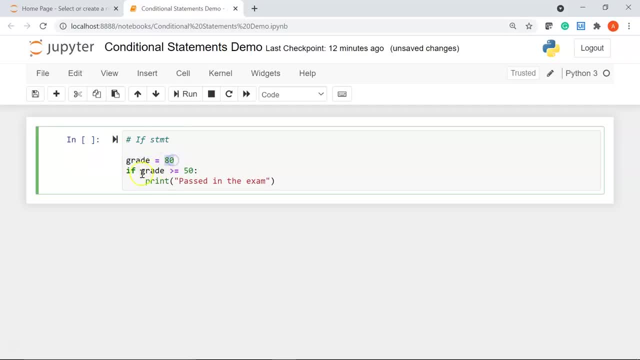 here I have already defined my grade to 80. So this if statement or this if statement or the if condition will check whether 80 is greater than or equal to 50. Now, this is true, Then my print statement gets executed. Let me run it and show you the result There. 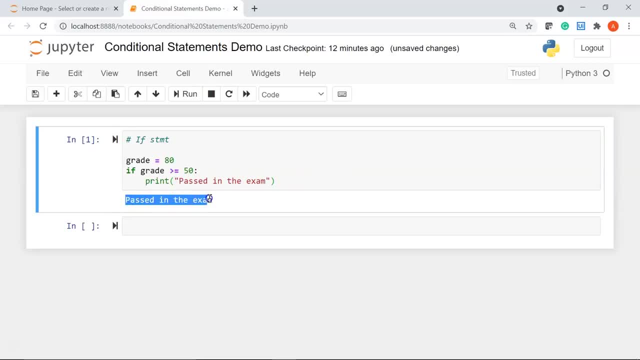 you go Here, you can see we have our printed message as passed in the exam, because 80 is greater than or equal to 50. But what if I change this to, let's say, 30? If I run this, there is no output here. 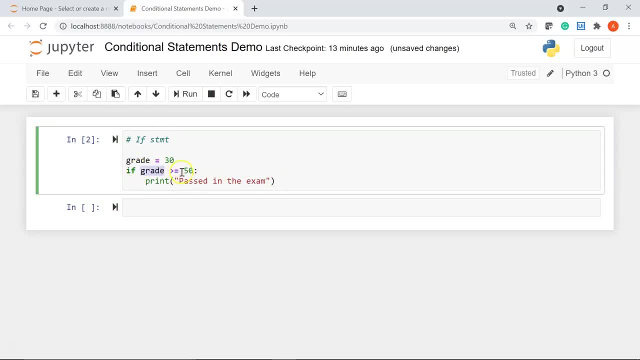 The reason being 30 is greater than equal to 50 is false, so my print statement did not execute. okay, now, if you want, you can also print another statement outside the if condition. i'll give the message as execute statement after if. one thing to remember that. 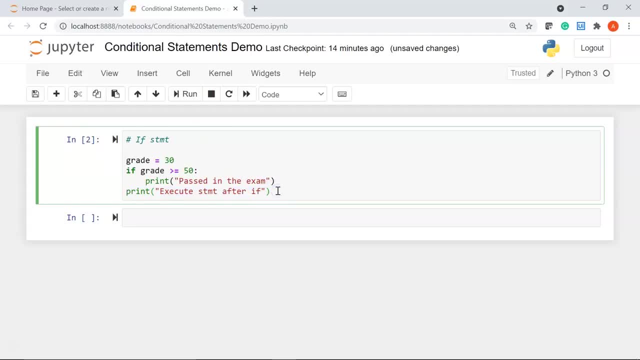 this print statement is outside the if condition. so if i run it, only my last print statement gets executed, which is outside the ifs condition. okay, now let's write another simple if statement. now, this time we are not going to define the grade value or pre-define the grade value here. 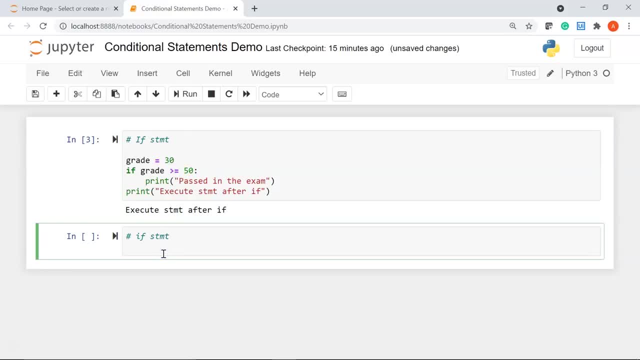 we are going to take the grade value as an input. that is a user input. so i'll write grade equal to. now. the way to take a user input is by using the input function. so first of all we need to convert our entry into an integer. so i'll write int function and inside that i'll pass in my input. 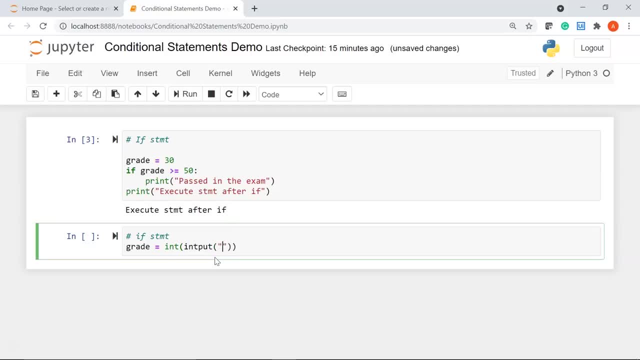 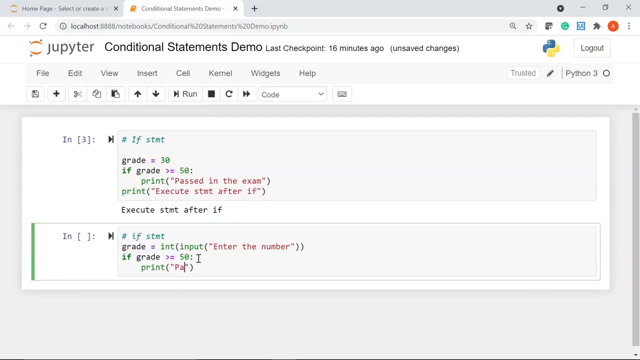 function. then i'll give my message as. enter the number. all right, so this statement will take the number from the user. now i'll write my if statement. if grade is greater than equal to 50, then it won't give a space here. let's delete the space, then i'll write: print: you have passed in the exam, okay. 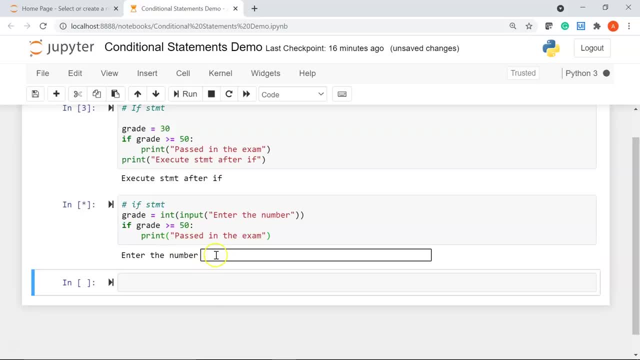 let's run it. you see here my program is asking for the user input. it says: enter the number. i'll give my number as, let's say, 60. if i hit enter, that gives me the result passed in the exam. now let's run it again. this time I'm going to give: 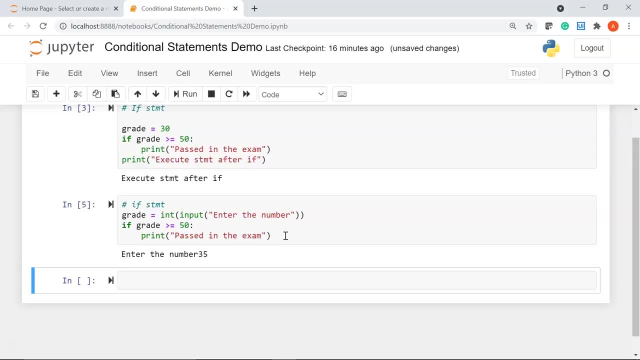 as, let's say, 35. if I run it, there is no output here, the reason being our grade 35 is not greater than equal to 50, so our print statement did not execute. all right, okay, now let me give a space here. we'll run it again, and this time we'll pass our grade as, let's say, 75. let me run it. 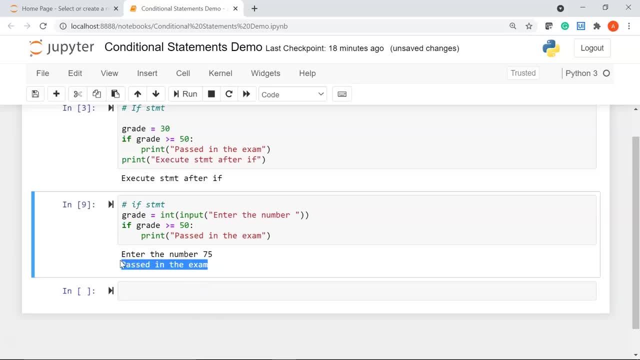 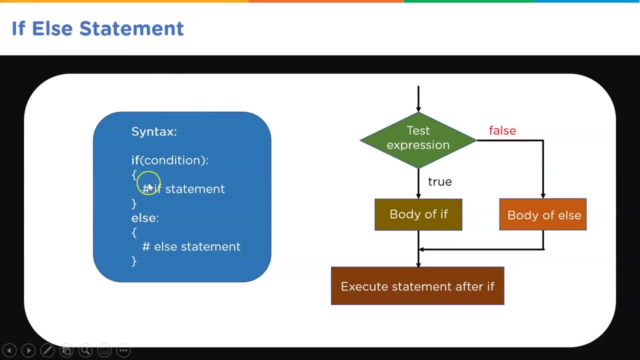 you can see here it gives me the message passed in the exam. now, moving to our next statement. we have the if else statement. so this is how the syntax of if else statement looks like. so first you have the if condition, followed by a colon. if this condition evaluates to true, then we: 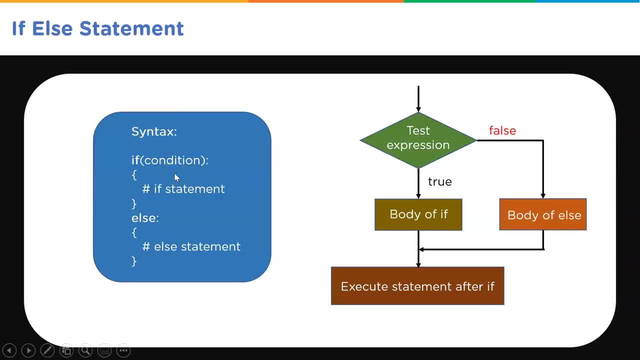 examine the if condition and if this condition evaluates to true, then we examine the if condition, execute the list of statements that are present inside this if condition. else we have the else block here. if this condition returns false, then we execute the list of else statements. so here is the flow of how the if else statement executes the different. 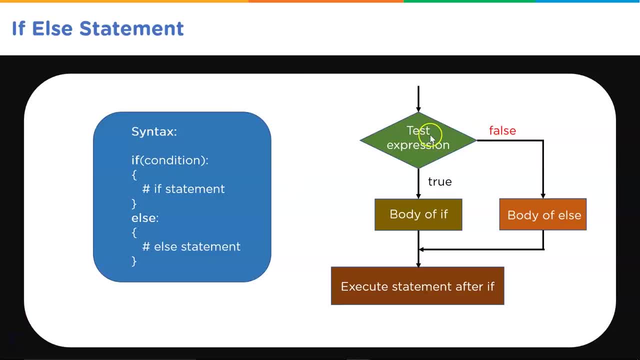 statements. so first we check the test expression. if that evaluates to true, then we have the body of if, and if it is false, then we have the body of else, and later there are any statements that are present outside the if else block, we'll execute those statements. now let's head over to our jupyter. 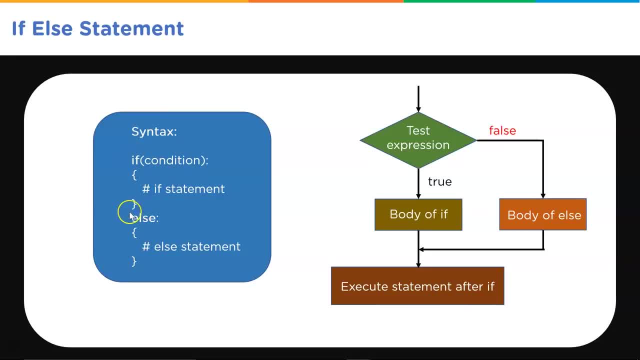 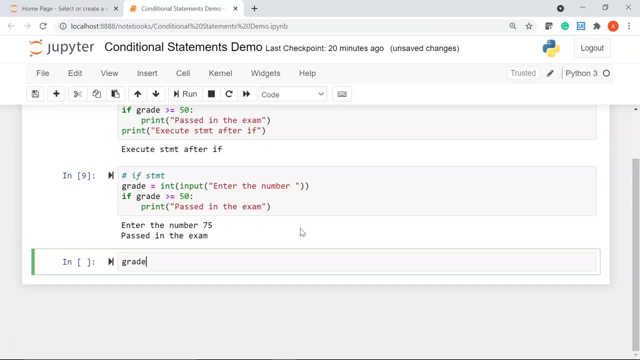 notebook and we'll see how the if else statement works by example. okay, so here i'll show you another example of using two if statements. so i'll define my grade as 40, i'll write: if grade is greater than equal to 50, then we'll print. 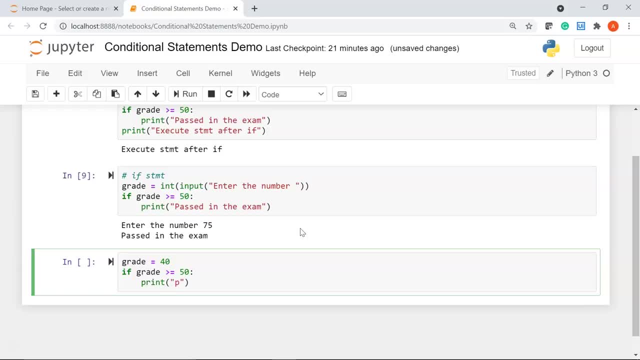 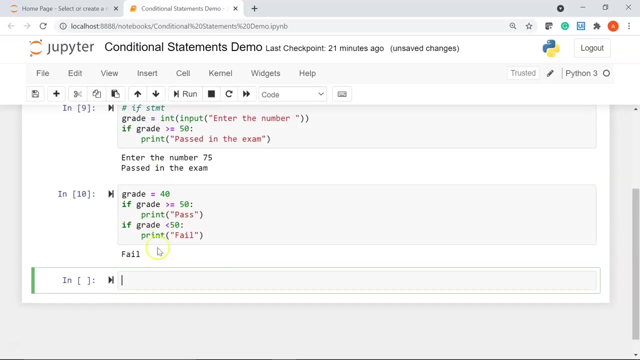 let's say pass, then i'll write another if statement. i'll say: if grade is less than 50, then we'll print fail. now, here i'm using two if statements. let me run it. you see, here i have my result as fail, the reason being our grade 40 is less than 50 and hence it has printed fail. 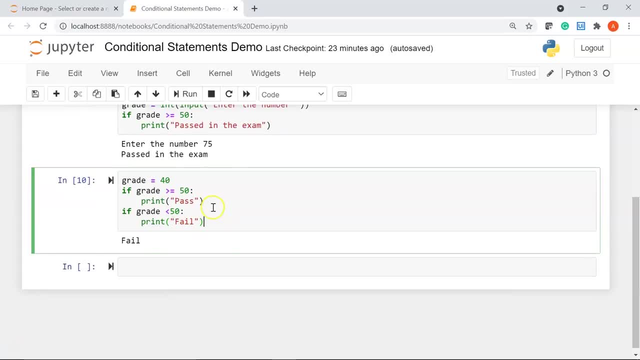 now, instead of using two if statements, you can use the if else statement. so in this case, we'll have our if statement checked for if grade is greater than equal to 50 and hence it has printed. if this is true, then we'll print whatever is there inside the if statement, but in case this evaluates, 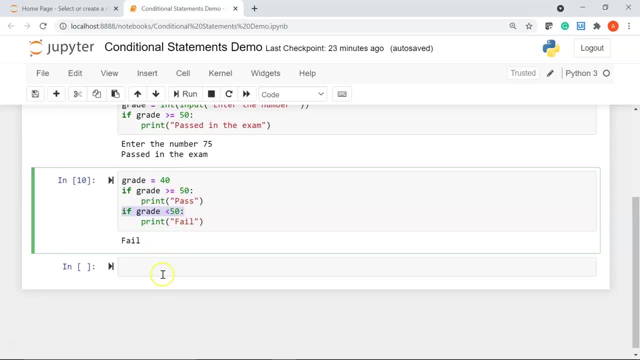 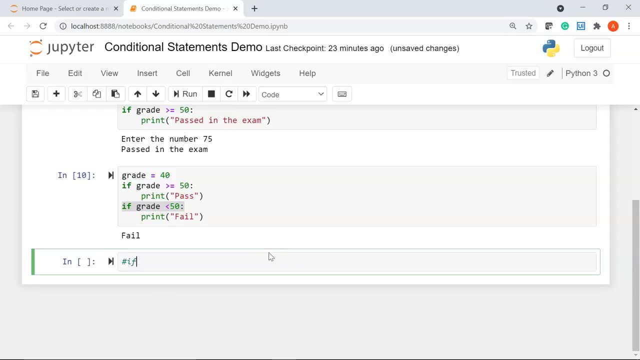 to false. we have another else block that we are going to write. let me show you how to write the false statement. so i'll give a comment as if else. okay, i'll say grade equal to 40I'll give a comment as if all else. OK, i'll say greed equal 40. 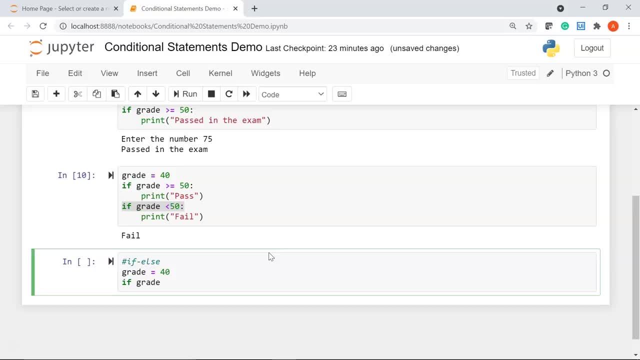 then we'll check. if they're faster than we're running past, then i'll check that info, that if i cancell it so then I'll check if the test data was better than that grade equal to 50. if you want toしてGo through E d on to, this must be completed done. force tests already need to need to be completed. 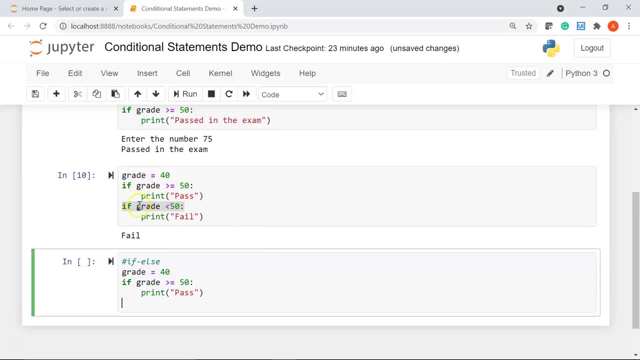 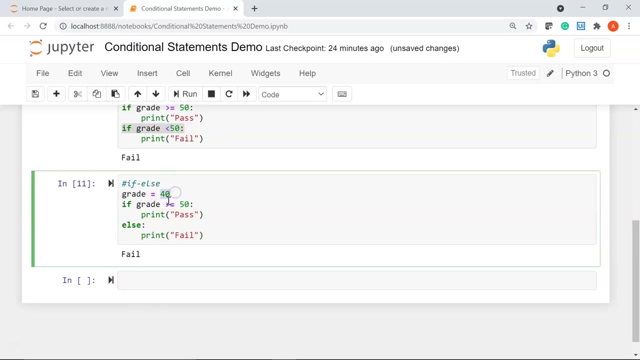 instead of using the if statement again, I'll write else, followed by a colon, and then I'll write print fail. make sure this fail is inside double quotations. if I run it, it gives me the result fail, the reason being: 40 is not less than repeat. 40 is not greater than equal to 50, so hence it has printed feel now instead of. 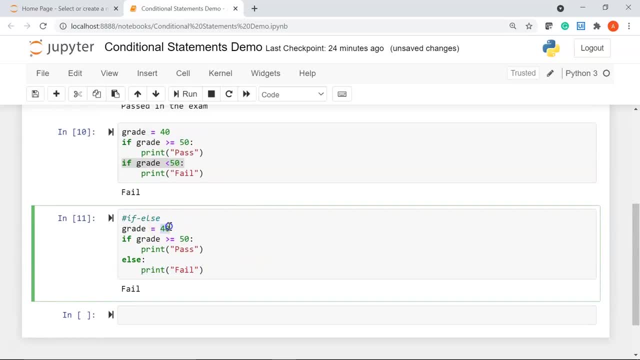 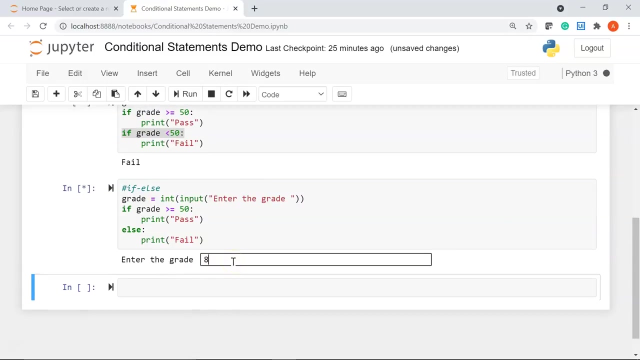 taking the value as 40, we can have the user give the input, so we'll use the input function. I will say: enter the grade, let's run it again. you see here my program is asking for the user input. let's say I'll give 80, will run it. it says pass because 80 is greater than. 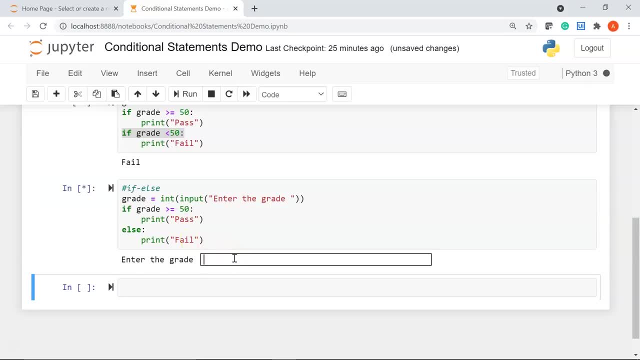 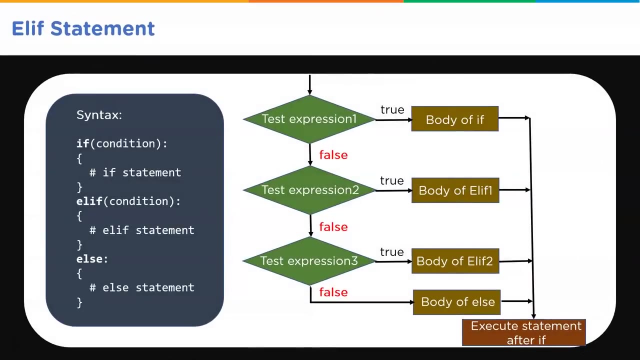 equal to 50. let me run it again this time. let's say I'll pass my grade as 45 will run it. it gives us fail. all right. now, moving to our next conditional statement, we have the elif statement. now this is how the syntax of elif statement looks like. so here, first we have the if condition Knife, the 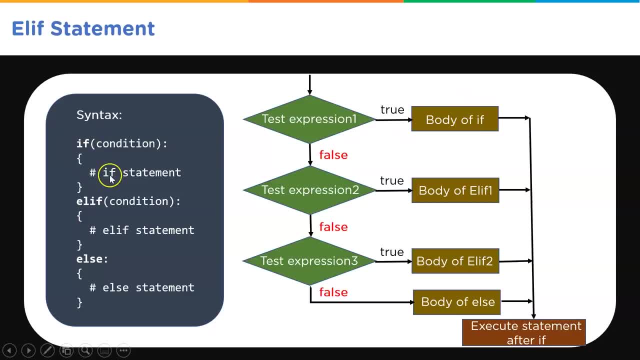 if condition evaluates to true, we have the body of. if that is basically a set of statements. now, if the first test expression of the condition evaluates to false, then our elif condition gets executed. now if I Elif condition is true, then we have the body of editor. so this is the elif statement body. 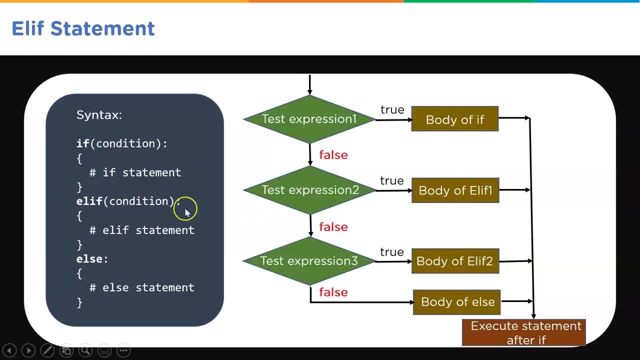 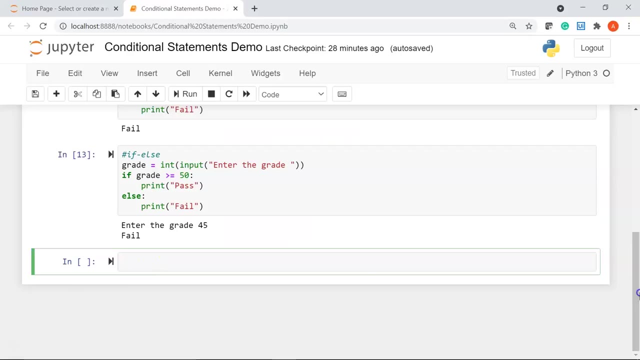 finally, if the Elif condition also evaluates to false, then you can enter a. then we have the block of else statements. you can see here we have body of else and later if there are any statements outside this, if elif and else block, then those statements get executed. now we'll see this with the help of examples. okay, so here on my cell i'll give. 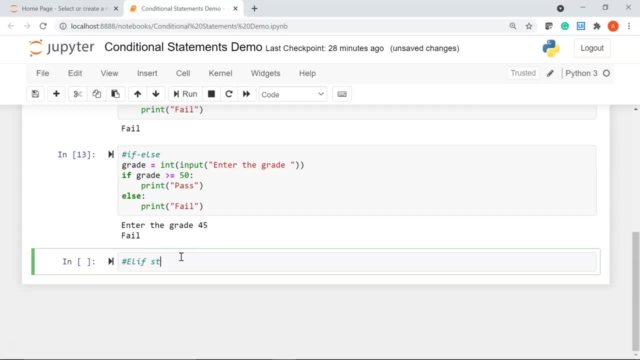 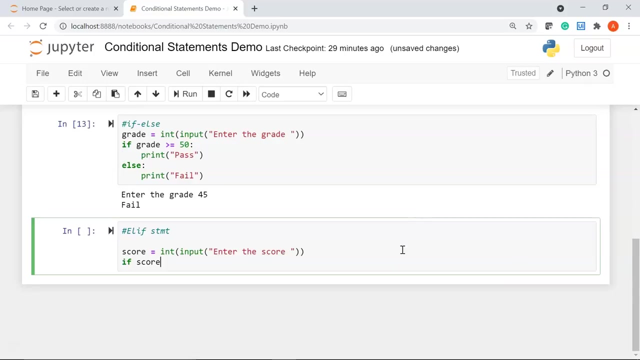 my comment as elif statement. okay, suppose i have a variable called score and this take the value as integer from the user. so i'm using the input function. i'll say: enter the score again, give a space. then i'll write my if condition. i'll say if score is, let's say, greater than 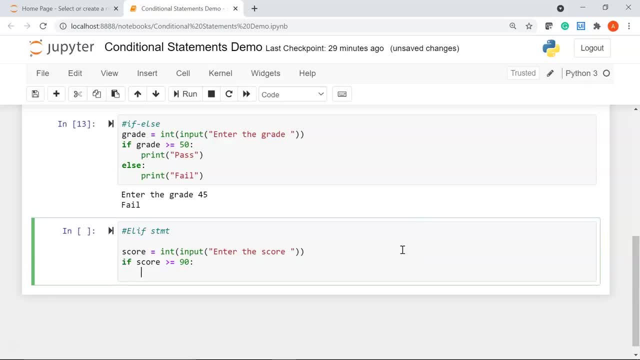 equal to 90. give a colon, then we'll print our message as passed the exam with, let's say, a grade. i'll just copy this statement, because we are going to print similar statement below as well, and now i'll have my elif condition. i'll write: 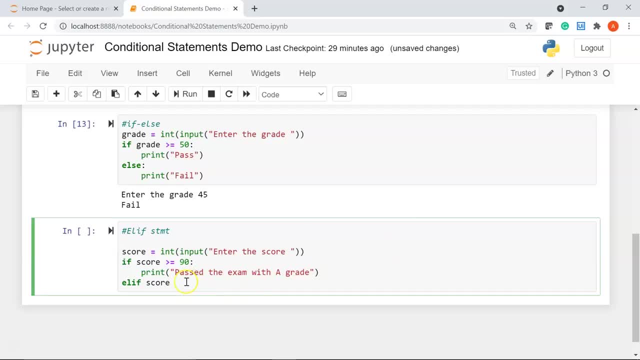 elif. elif is actually else. if score is greater than equal to, let's say, 75, i'll give a colon. will print pass the exam with B grade. then I'll again have my elif statement I'll write. if score is greater than equal to, let's say, 60, will print pass the exam with C grade. 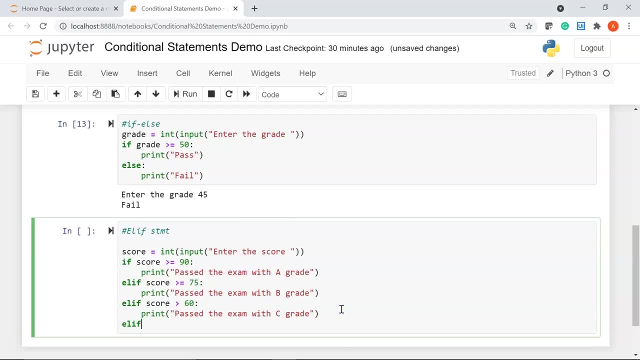 next let's write another elif condition. I'll write elif: if score is greater than this should be greater than equal to. okay, it's greater than equal to, let's say 40. then we'll print pass the exam with D grade and finally we'll have the. 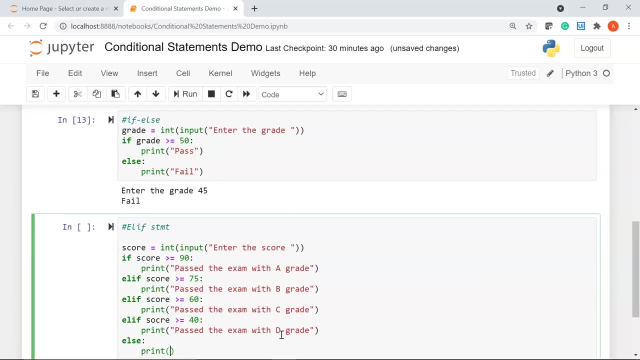 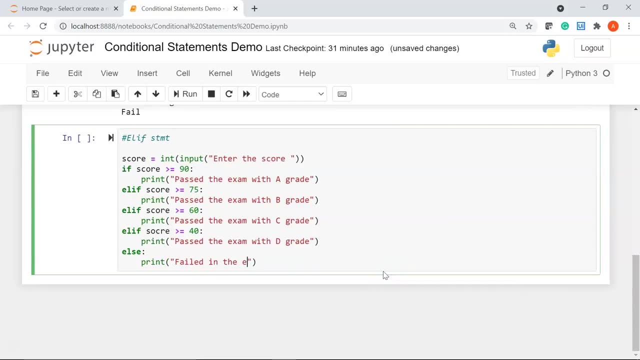 else condition I'll write print. let me just scroll down. failed in the exam. okay, so this is how you write a elif conditional statement. so first I am taking the user input of the score, then I'm checking. if score is greater than equal to 90, I am displaying. 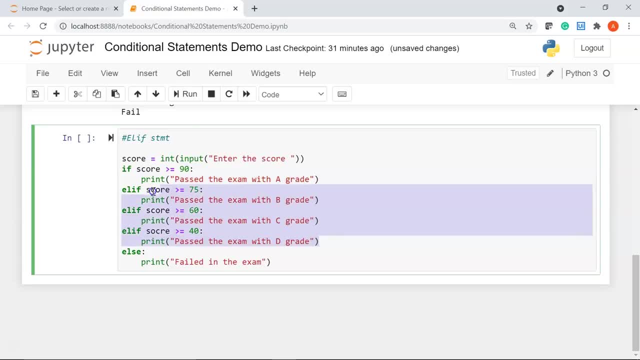 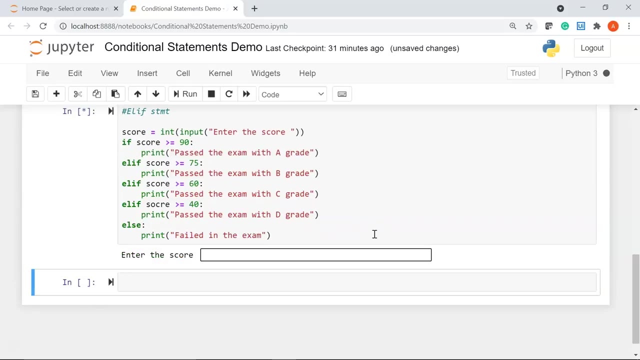 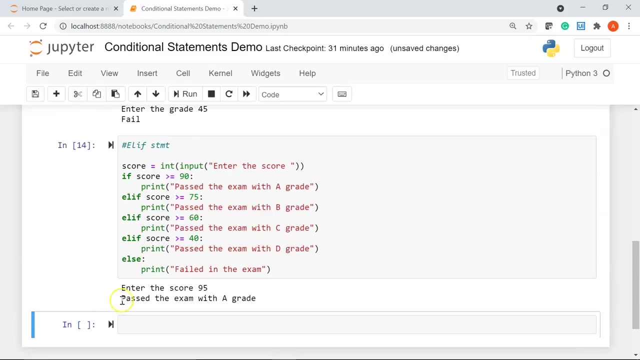 my message has passed the exam with a grade. then I have a list of elif statements to check for different scores. if all these evaluates to false, I am having my else statement printed. let's run it okay, so we'll try out different scores. let's say someone scored 95 if I run it so that candidate has passed the exam with. 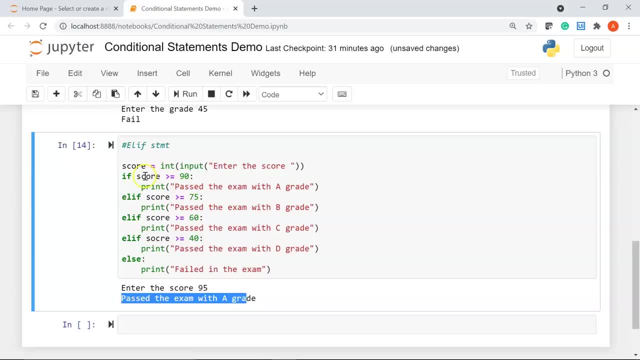 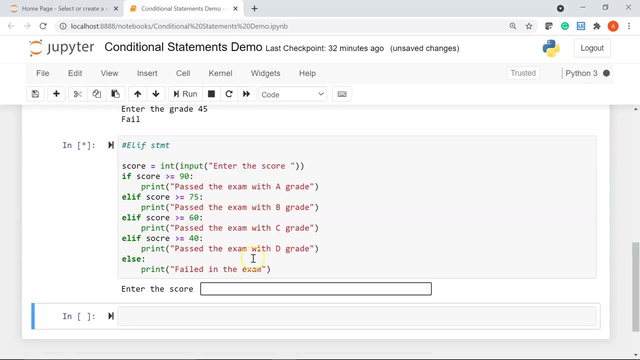 A grade because someone scored 95, so that candidate has passed the exam with E grade because, if you see the condition, my score 95 is greater than equal to 90 and hence we have pass the exam with a grade. as the message run it again, let's say i have 80 if i run it. 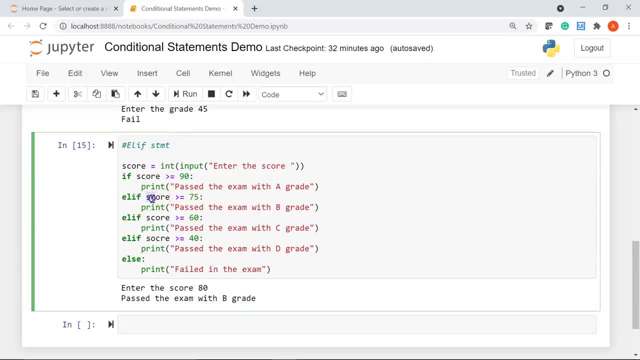 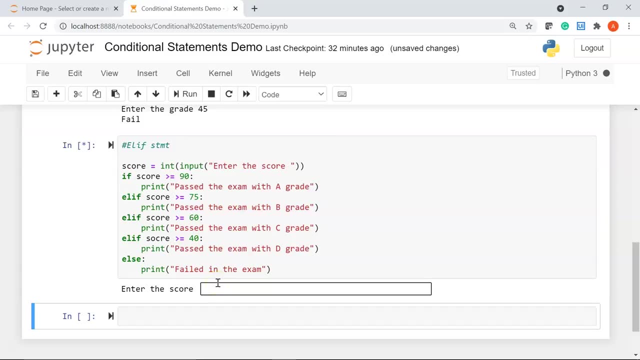 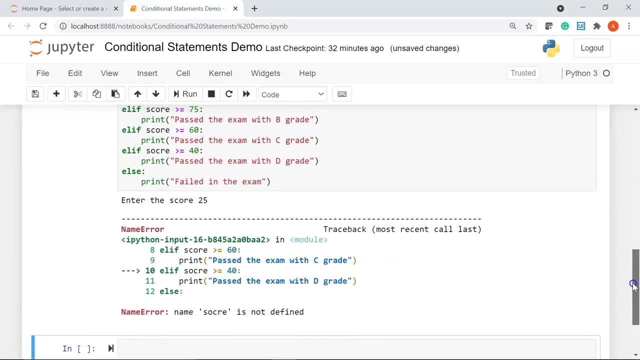 it says pass the exam with b grade, the reason being 80 is greater than equal to 75 and hence we have this message printed. let's run it again. suppose someone scored, let's say, 25. if i run it, okay, it throws me an error. it says: name score not defined. okay, so this should be. 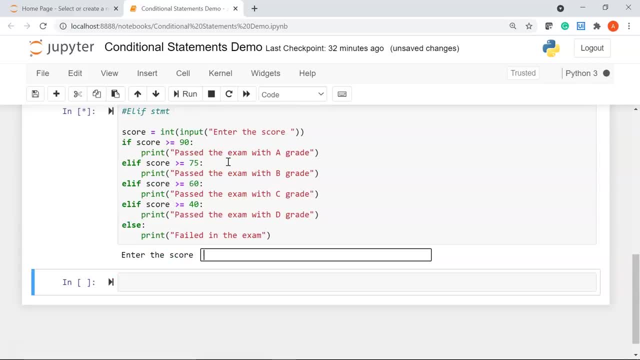 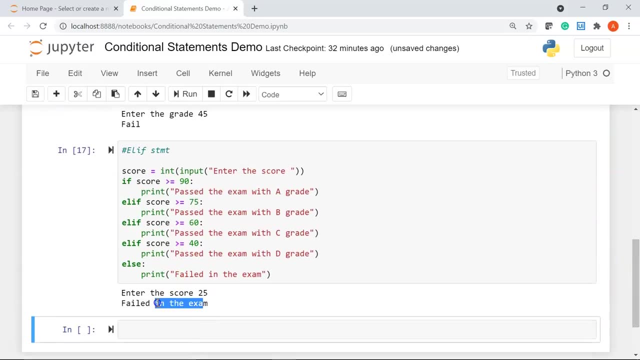 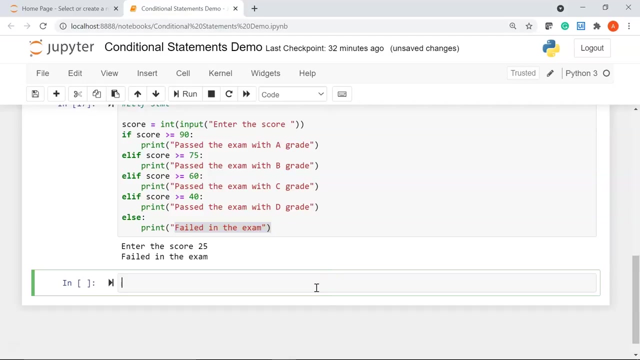 score. actually here there was a spelling mistake. i'll run it. i'll pass my score as 25. it gives me failed in the exam, the reason being my score 25 is less than equal to 40 and hence we have failed in the exam. cool, now you can also use a for loop and then have a list of if else, block or if else. 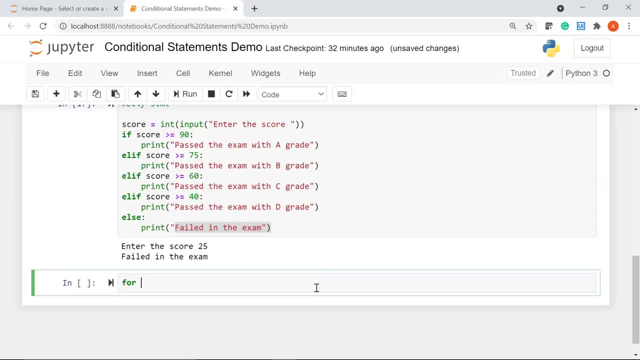 statements. let me show you how to do it. suppose i write for x in, i'll use the range function. i'll go till 10, which means from 0 to 9, then i'm checking if my x is greater than equal to 90, and hence we have a list of if else block or if else statements. 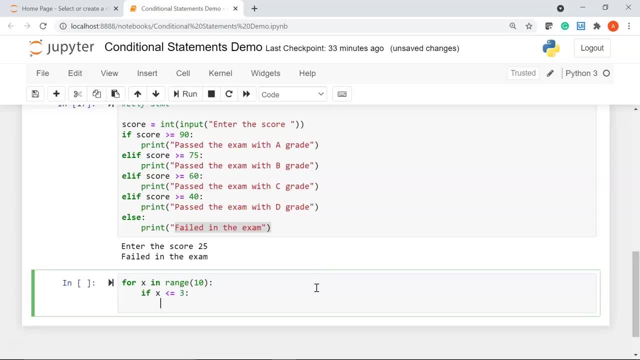 less than equal to 3, i'll print. x is less than or equal to 3. okay, now we have the elif statement. if elif x greater than 5, i'll print. x is greater than 5, then we have the else condition will print. let me just scroll down. 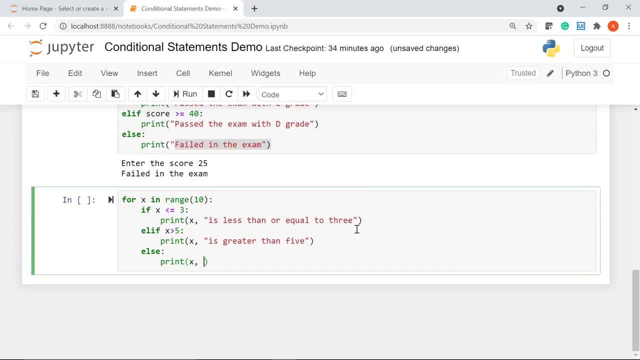 we have set three go feed for a increase interval undefined, i'll print x must be 4 or 5, okay, so here i've used a for loop and i'm checking for each iteration from 0 to 9, and then we have a set of- if 11 else- statements. lets run it. there you go, you. 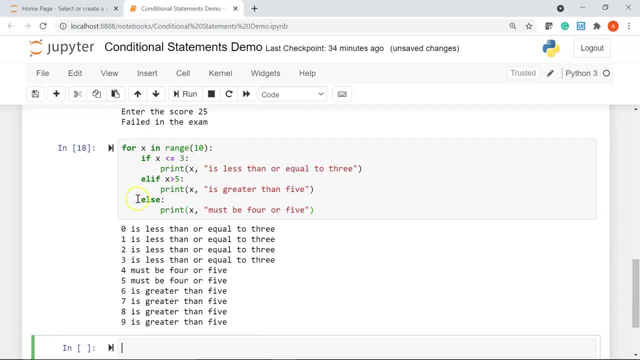 see the output here. so first, in my range i have zero, so it will check if zero is less than equal to three, which is true. so it has printed zero is less than or equal to three, so it will go till three, and then when four comes, it will check if four is greater than five. now this is also false. 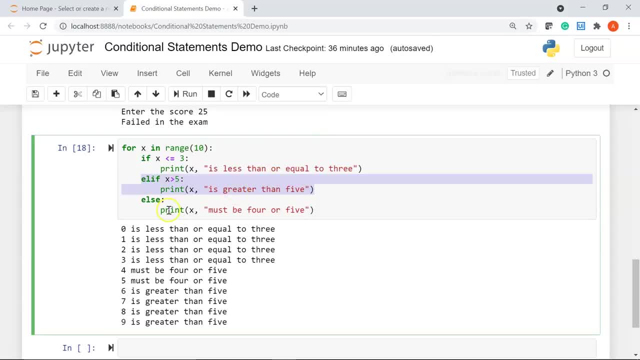 so it will skip executing the lf statement and it will print whatever is there in the else block, which is: four must be four or five. so you can see the message here: four must be four and five. similarly, for five also, the same message will be printed, the reason being: five is not greater than. 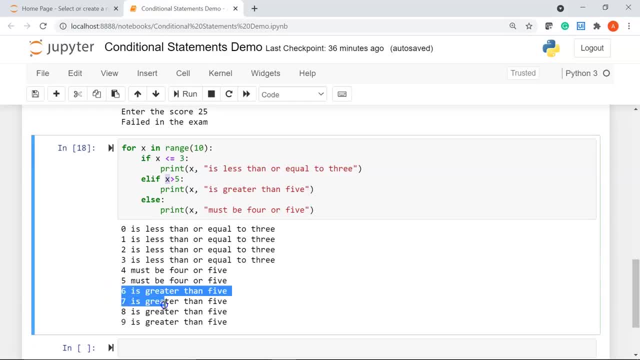 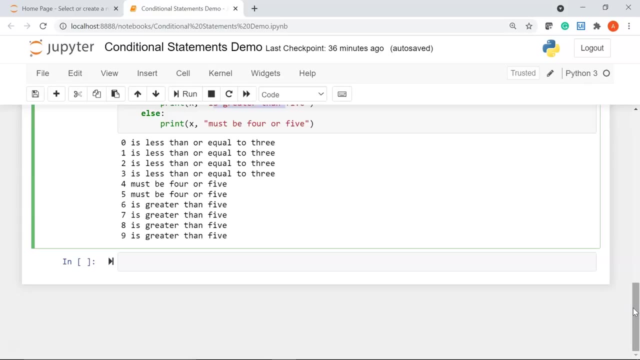 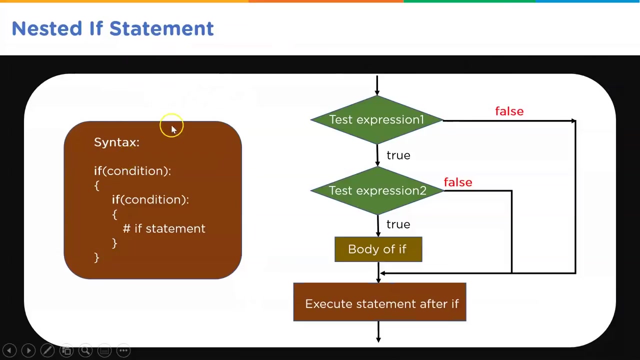 five. and then for the rest of their numbers, from six to nine, we have: six is greater than five, seven is greater than five, eight is greater than five and nine is greater than five. all right now. moving ahead, next we have the nested if statement. so here is the syntax of nested if. so you have the if. 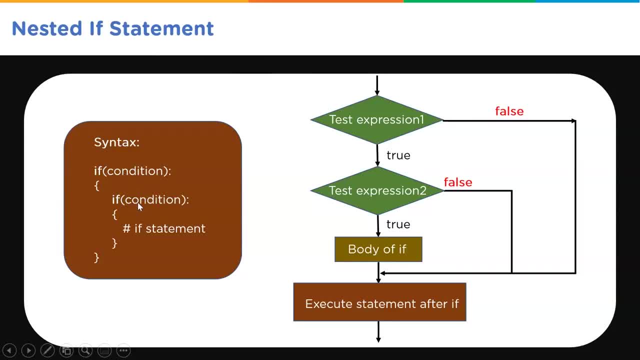 condition, and inside the if condition you have another if condition, and hence it becomes the nested if condition statement, and inside this condition you have the list of statements, or the blocks of statements. so here is how the flow chart, or the flow diagram, looks like. first we are evaluating the expression one, which is this: 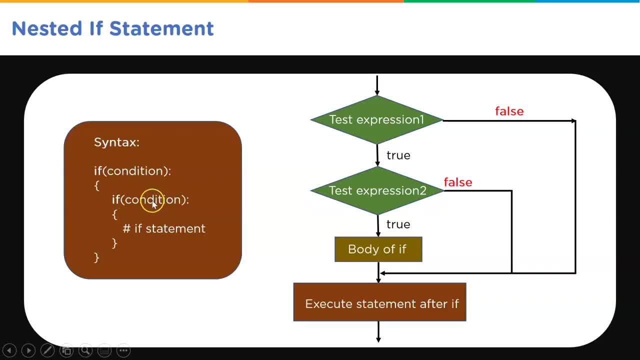 condition. if it is true, we are going inside and checking the second condition. if that is also true, then we are running the body of which is this part of the syntax, and later, if there are any statements that are present outside the if condition, we are executing those. 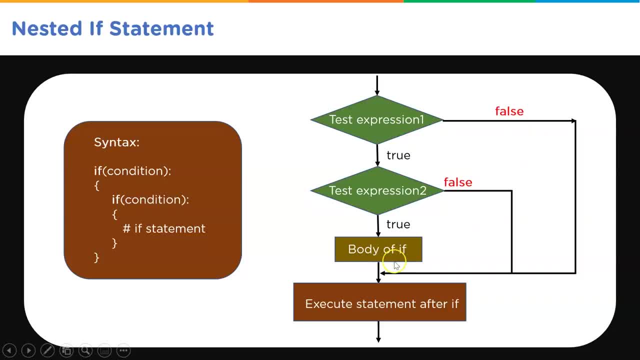 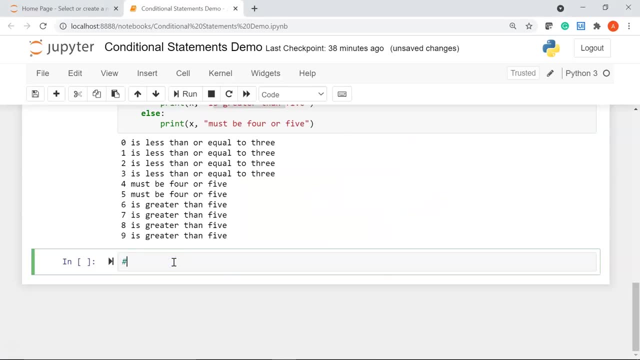 so in case the first test expression evaluates to false, we are coming outside and directly printing whatever is there outside the if condition. let's see this with the help of an example. okay, so i'll give my comment here as nested if cool. so first of all i'll. 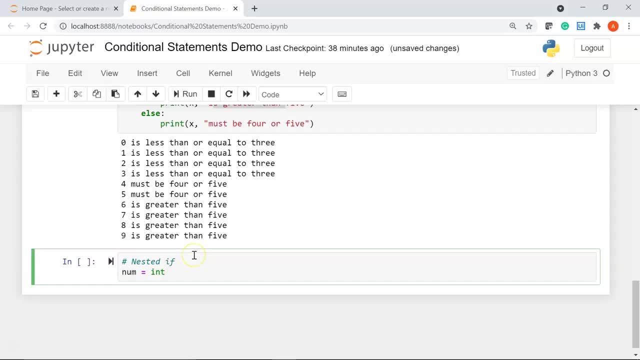 declare a variable called num. now this num will have a user input value. so i'll write input, enter the number and then i'll have my first if condition. i'll say if number or num is less than 250, i'll give a colon. then we'll use the print statement: num is smaller than 250.. 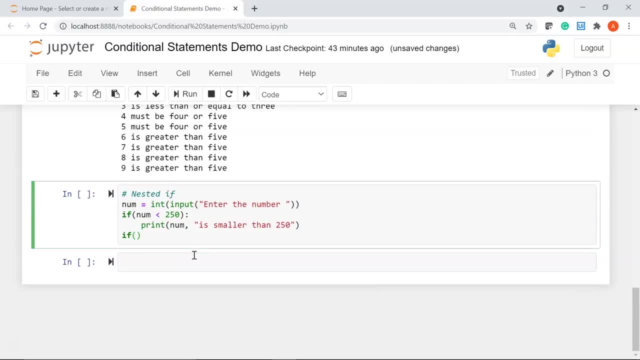 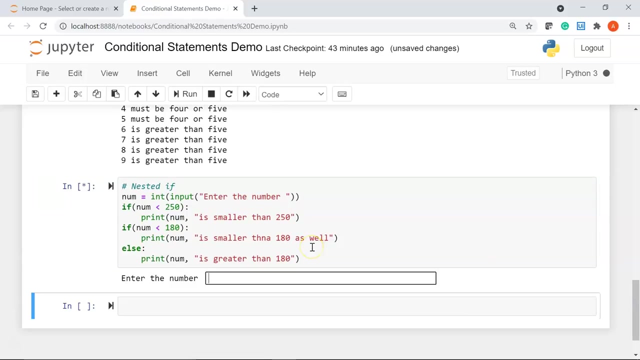 i'll write my second if statement and we'll check if num is less than 180 and we'll print num is smaller than 180 as well. finally, i'll have my else statement as print, say, number is greater than 180. all right, let's run this, and first we'll check with the number 100. okay, there you go. 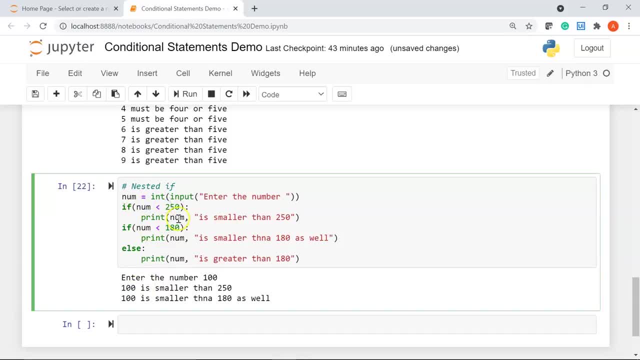 so here i'm checking whether 100 is less than 250, which is true, so we have printed: 100 is smaller than 250.. again, we are checking if 100 is less than 150. so we are printing 100 is less than 250. 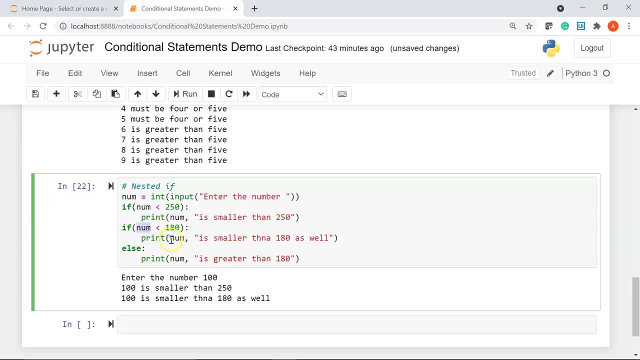 again. we are checking if 100 is less than 150. again we are checking if 100 is less than 250.. we are checking if 100 is less than 180, which is true again. so we are printing: 100 is smaller than 180 as well. there's a spelling mistake. okay, now let's see. for let's say 150 again. we have. 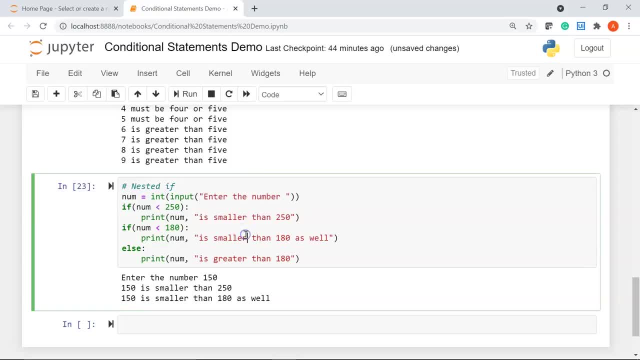 150 is smaller than 250. 150 also smaller than 180. let's run it this time. let's say, we'll pass 300. okay, you can see our result here: 300 is less than 250 is false, so we'll skip printing this again. we'll check whether 300 is less than 180, which is false again, so we'll skip printing this. 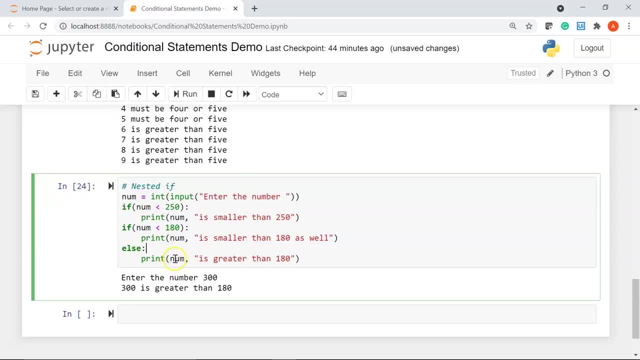 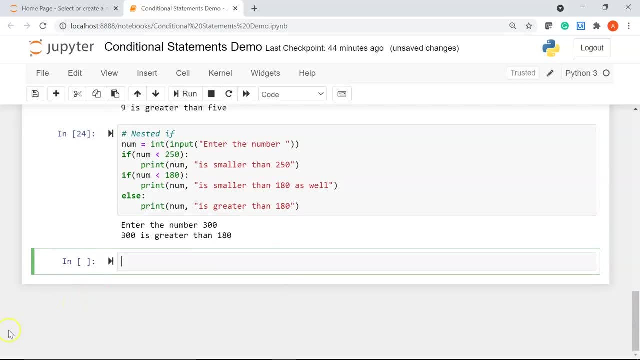 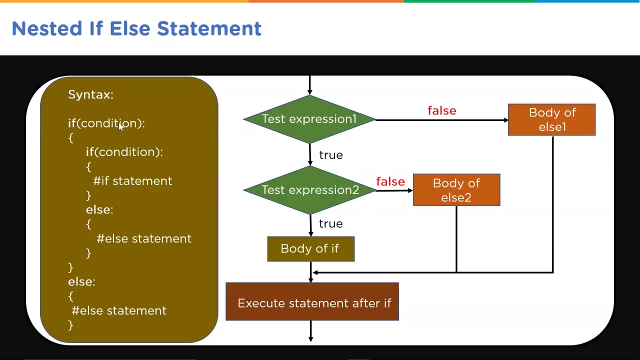 statement as well. we'll only have our else block printed, which is 300 is greater than 180. okay, now coming to the final section where we'll see about nested if else. so here you can see we have the syntax for nested if else statement. so we have an outer if condition and inside that we have another if condition. 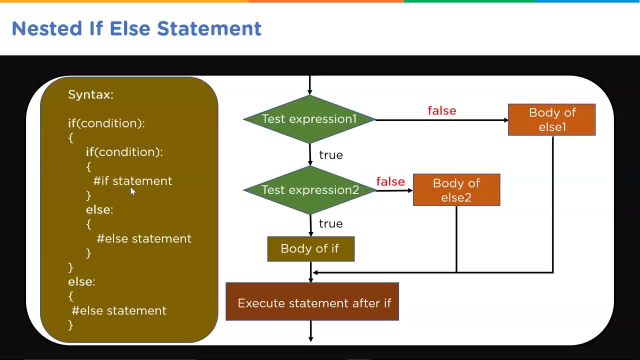 then we have the list of statements or the body of the if condition. if this is false, then we execute the else part and after that we also have an outer else statement. so this is how the flow diagram looks like. we'll check for the test expression 1. if that is true, then we'll go. 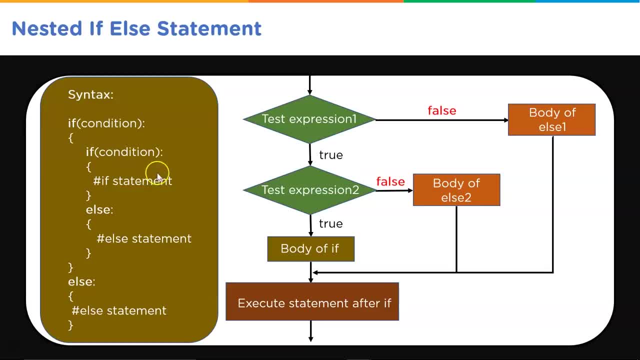 inside and see the test expression 2, and if that is true, we'll execute the body of if statement, which is this part of the syntax. then, if these are false, then we'll see the body of else 1. if the second expression is false, then we go to the body of else 2 and after that, if there are 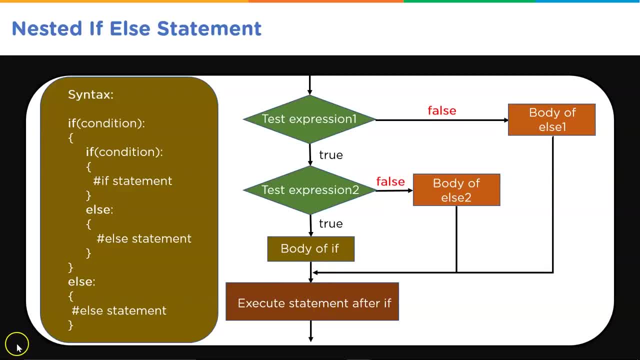 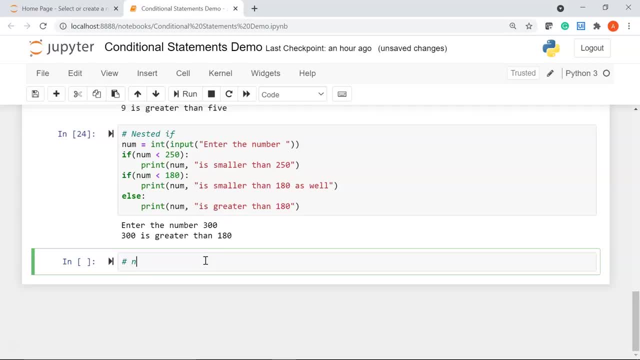 any more statements, we'll execute them as well. all right, we'll see an example here, so i'll give my comment as nested, if else okay. so i'll declare a variable a, which will take a user input of type integer. i'll say: enter the null. i'll write if a is less than 50. 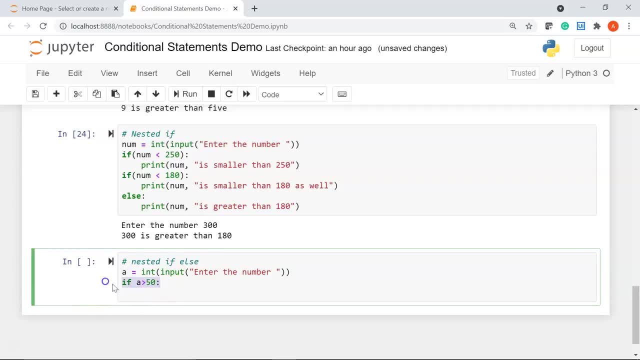 so this is my first if condition. if this is true, this should be less than 50. okay, so if my first if statement is true, then we'll check for the second if statement, which is, let's say, if a modulus 3 equal to equal to 0, which means if the 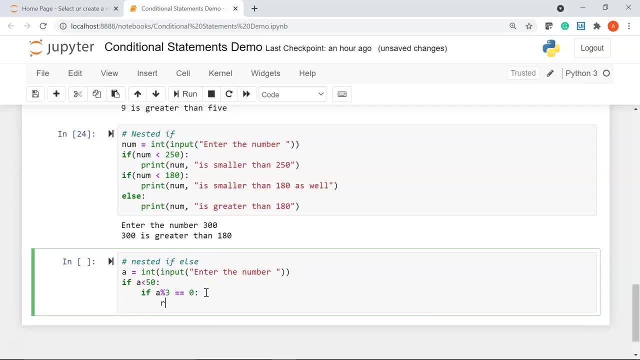 remaining if statement is true, then we'll check for the second if statement, which is, let's say, if the remainder of the division is 0, then we say print a is divisible by 3 and is less than 50. okay, then we have our render of the division is 0, then we say print a is divisible by 3 and is less than 50. okay, then we have our 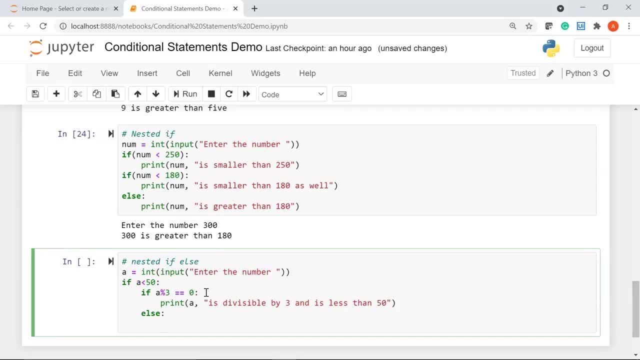 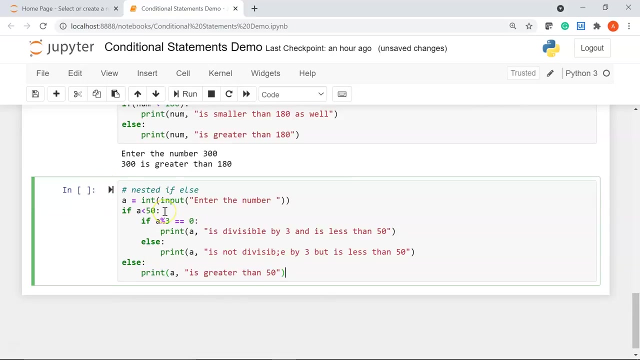 our else statement, as else print my number a is not divisible by 3 but is less than 50. finally, I will have my last else statement where I will print my number a is greater than 50. ok, so this is how you write a nested if else statement. so I am taking my number as a user. 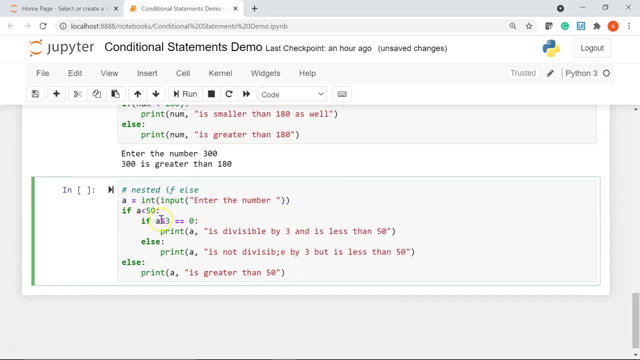 input. first I am checking if that number is less than 50. if that is true, I am again checking if that number is divisible by 3. if it is divisible, I am printing my message, as the number e is divisible by 3 and is less than 50. 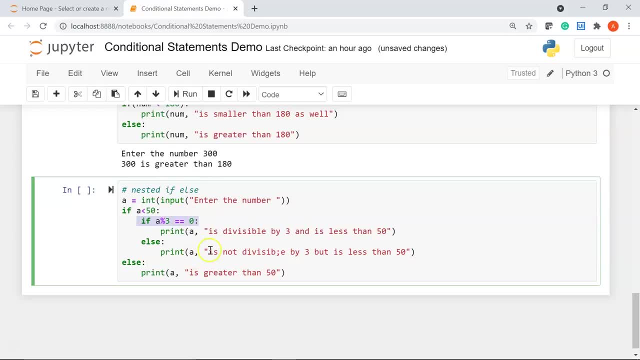 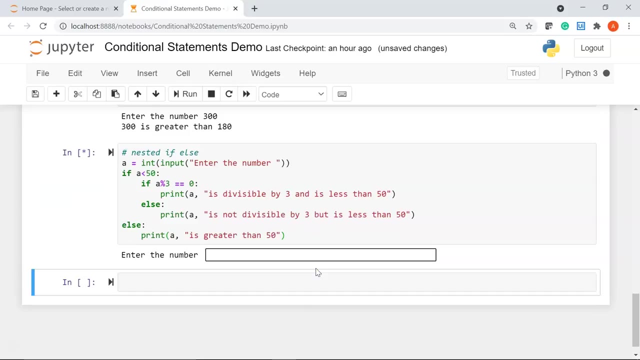 if this is false, I am saying the number e is not divisible by 3, but it is less than 50. else I am saying the number is greater than 50. let's run this and we will try out different examples. let's say, I will say: 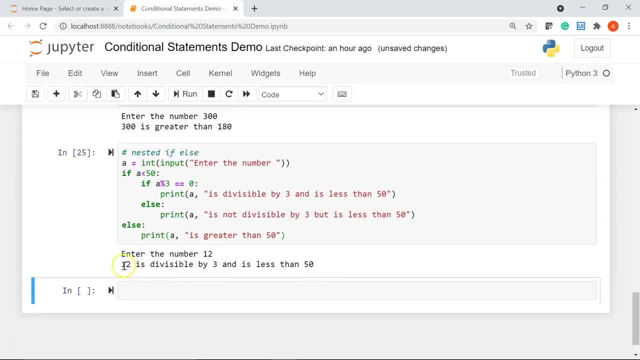 my number is 12. my message is: 12 is divisible by 3 and is less than 50, which is this part of the code. so my number, 12, is less than 50. this is true. then I am again checking whether 12 is divisible by 3. 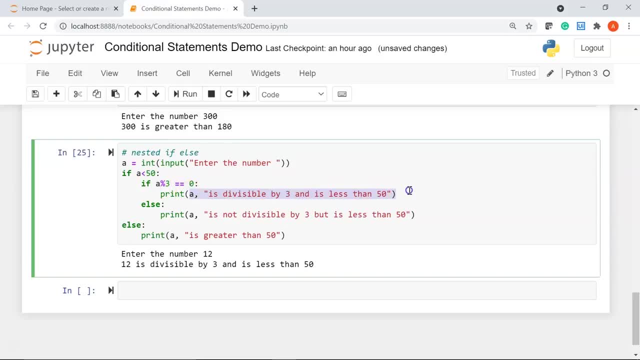 it evaluates to true and hence we have this result printed. ok, let's say, this time I will say 30. so I have my message: 30 is divisible by 3 and is less than 50. let's run it again, and this time let's say we will say 72. 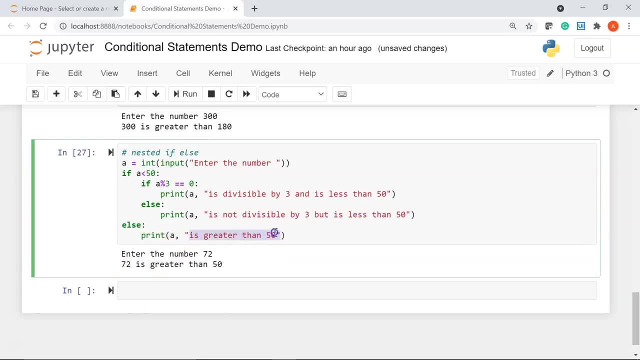 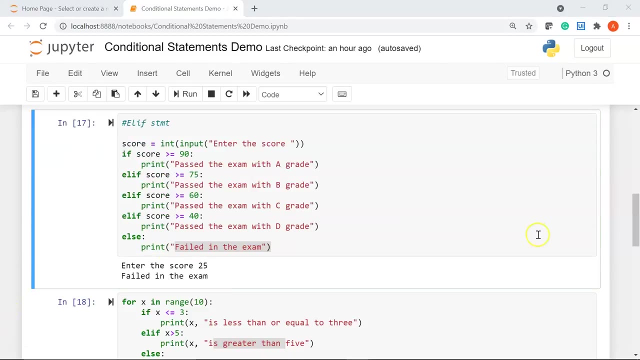 so here I have my message: 72 is greater than 50. the reason being 72 less than 50 is false. hence this part of the code is not executed. it will directly come to the else part, which says 72 is greater than 50. ok, 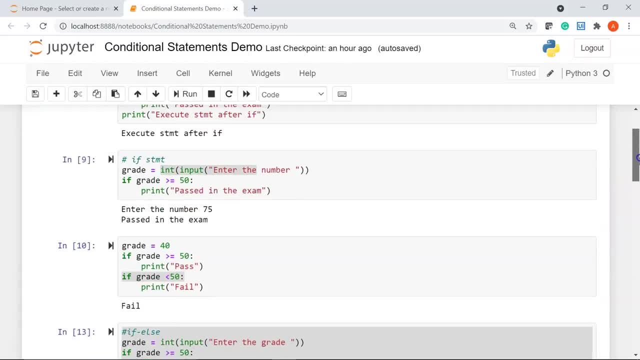 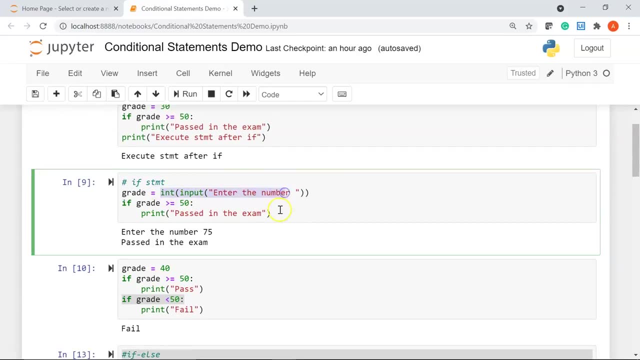 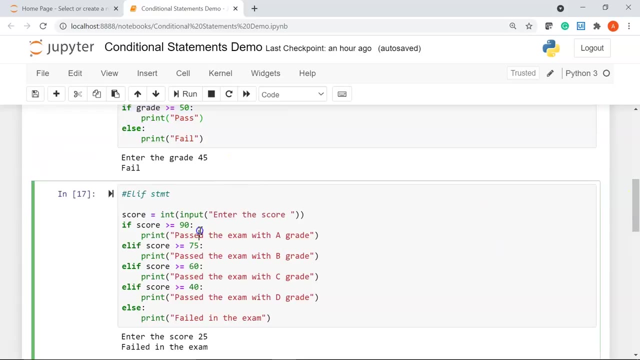 so that brings us to the end of this demo session on conditional statements in python. so first we learnt how to write simple if statement. you saw how to take inputs from the user. we also learnt how to write if else statement. then we learnt about elif statement. you also saw how to use for loop. 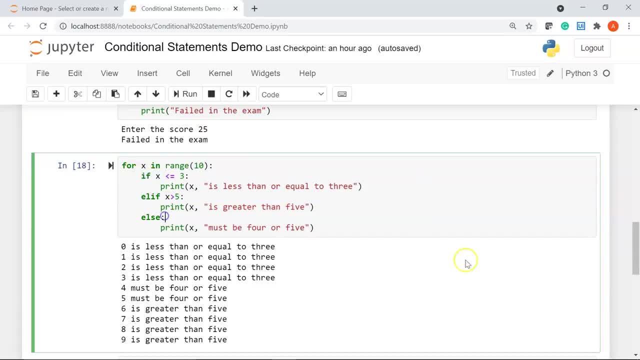 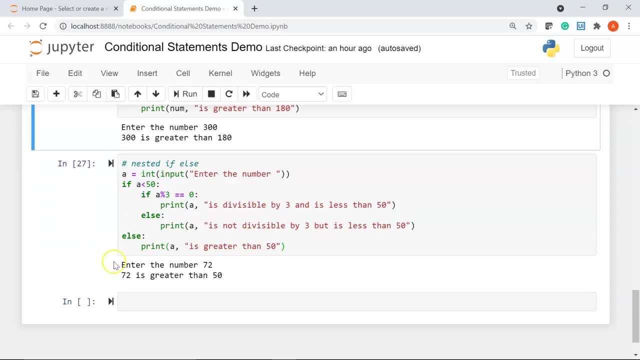 and inside that you can use your if statement, your elif, your else. later on we saw how to write nested if statements and finally we learnt how to write nested if else statements. so that brings us to the end of this video tutorial on conditional statements in python. 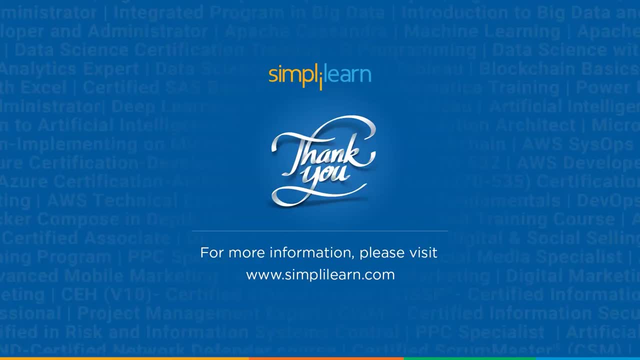 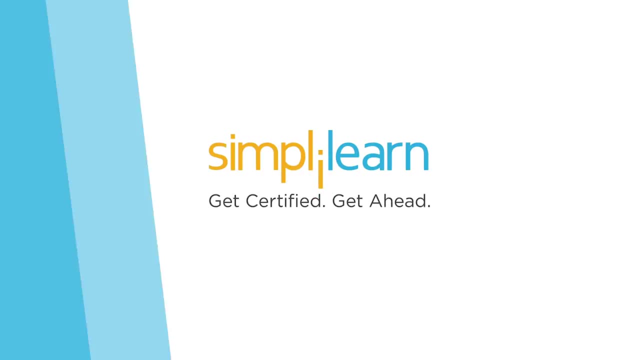 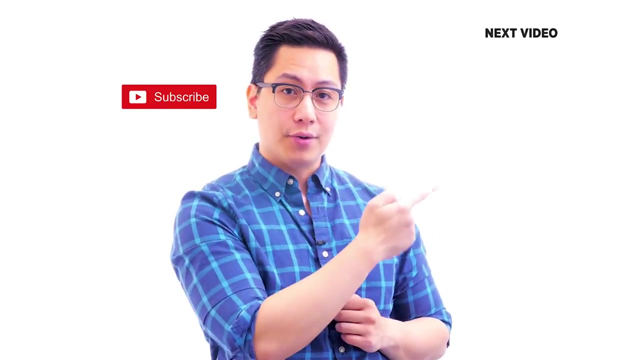 I hope it was useful and informative. If you have any queries, then please feel free to put them in the comment section of the video. Thank you for watching and keep learning.